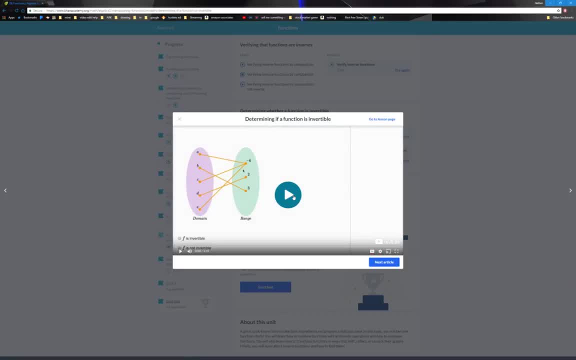 So now we have a quick video to watch and then we have an article, so we'll just watch that video. f is a finite function whose domain is the letters a to e. The following table lists the output for each input in f's domain. 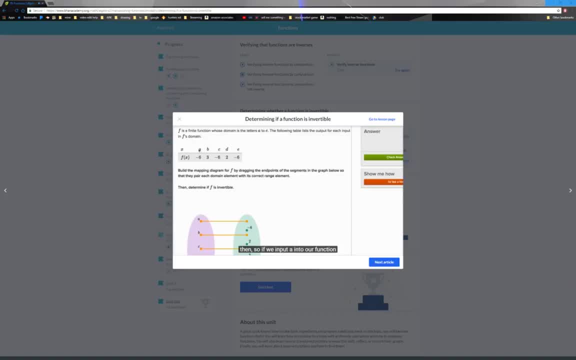 So if x is equal to a, then so if we input a into our function, then we output negative 6.. f of a is negative 6. We input b, we get 3. We input c, we get negative 6.. 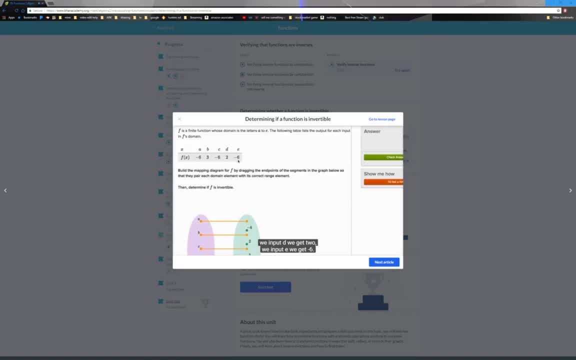 We input d, we get 2.. We input e, we get negative. 6. Build the mapping diagram for f by dragging the endpoints of the segments in the graph below so that they pair each domain element with its correct range element, Then determine if f is invertible. 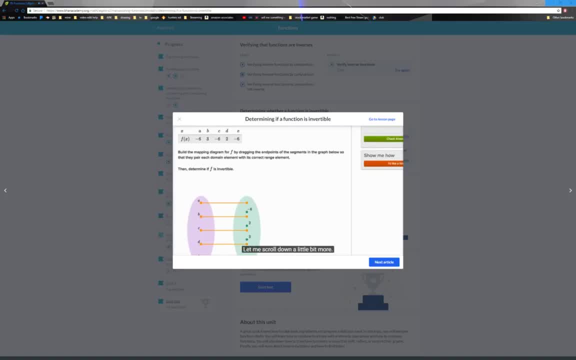 All right. so let's see what's going on over here. Let me scroll down a little bit more. So in this purple oval we're representing the domain of our function, f, and this is the range So the function is going to if you give it a member of the domain. 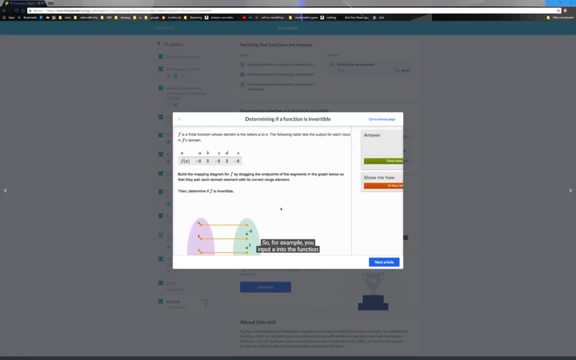 it's going to map from that member of domain to a member of the range. So, for example, you input a into the function, it goes to negative 6.. So a goes to negative 6, so I drag that right over there. 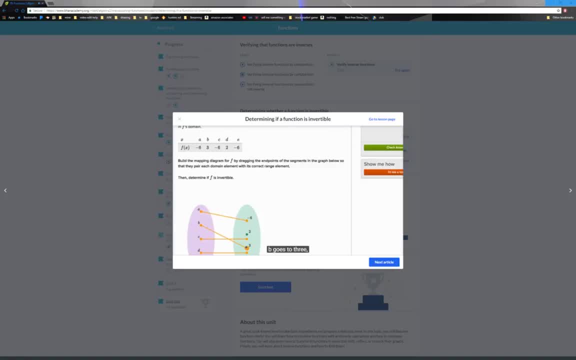 b goes to 3.. b goes to 3.. c goes to negative 6.. So it's already interesting that we have multiple values that point to negative 6.. So this is okay for f to be a function, but we'll see it might make it a little bit tricky for f to be invertible. 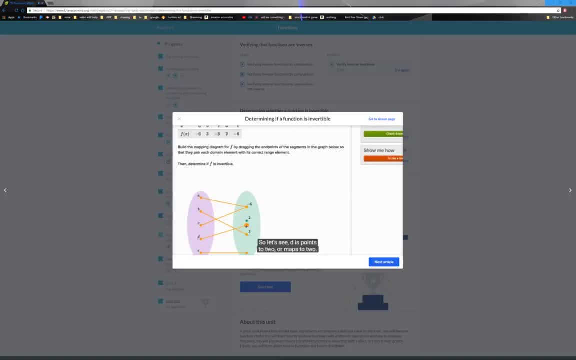 So let's see, d is points to 2, or maps to 2.. So you input d into our function, you're going to output 2.. And then, finally, e maps to negative 6 as well. e maps to negative 6 as well. 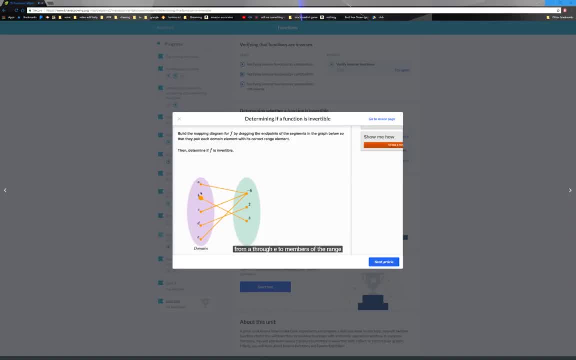 So that's a visualization of how this function f maps from a through e to members of the range. But let's also ask ourselves: is this function invertible? And I already hinted at it a little bit. Well, in order for it to be invertible, 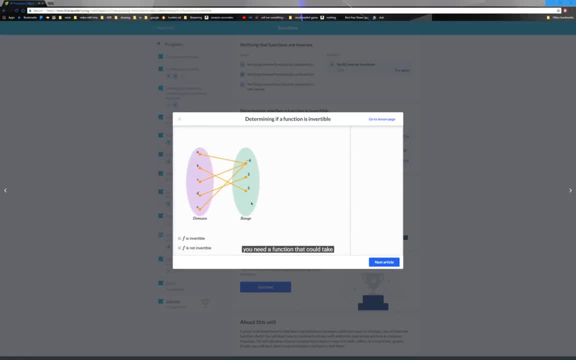 you need a function that could go from each of these points to that can do the inverse mapping. But it has to be a function. So if you input 3 into this inverse function, it should give you b. If you input 2 into this inverse function, it should output d. 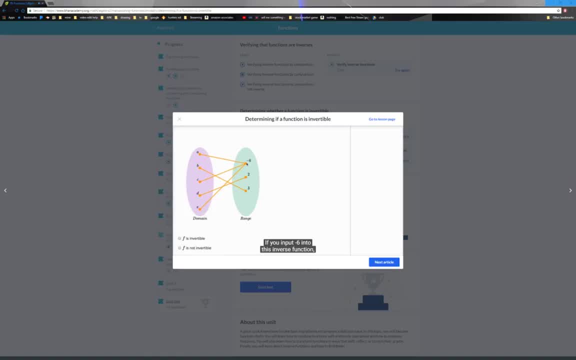 If you input negative 6 into this inverse function. well, this hypothetical inverse function, what should it do? Well, you can't have a function that, if you input a number, it could have three possible values: a, c or e. 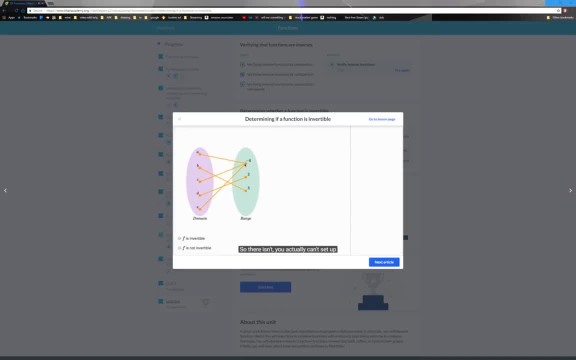 You can only map to one value. So you actually can't set up an inverse function that does this, because it wouldn't be a function. You can't go from input negative 6 into that inverse function and get three different values. So this is not invertible. 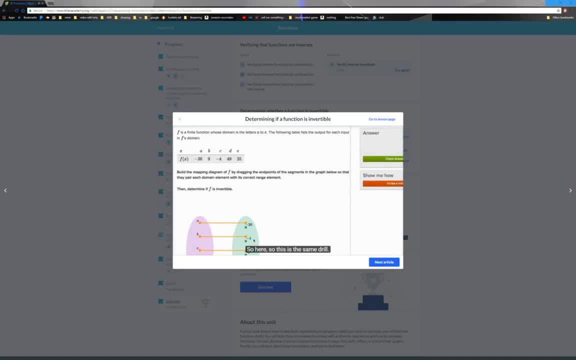 Let's do another example, So here. so this is the same drill. We have our members of our domain, members of our range. We can build our mapping diagram: a- maps to negative 36.. b- maps to 9. c- maps to negative 4.. 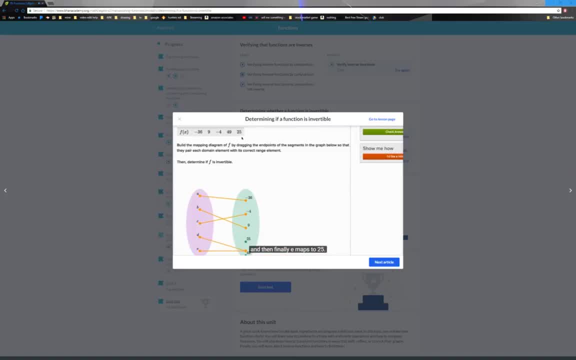 d maps to 49. And then finally, e maps to 25.. e maps to 25.. My bad f is a. finally, e maps to negative 6.. If you input 2 into this inverse function, what should it do? 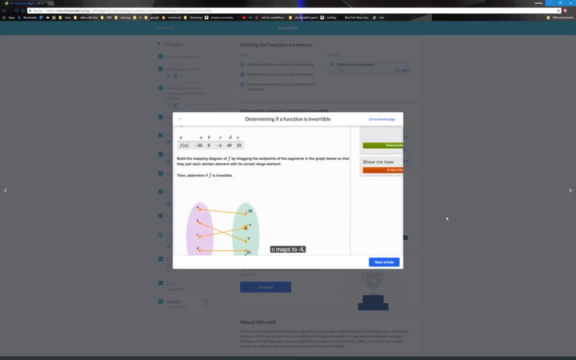 Three different values: c maps to negative, 4. d maps to 49. And then, finally, e maps to 25.. e maps to 25.. Now is this function invertible? Well, let's think about it. The inverse whoops. 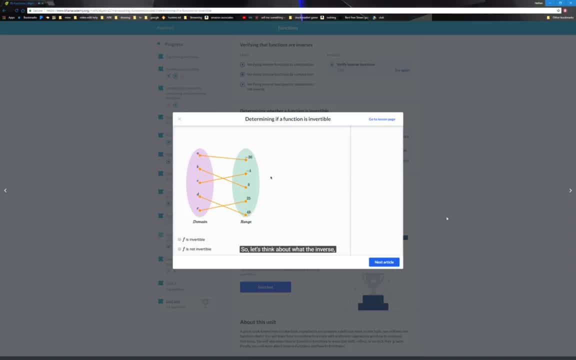 The what was it? d maps to 49.. So let's think about what the inverse, this hypothetical inverse function, would have to do. It would have to take each of these members of the range and do the inverse mapping. So if we input 49 into our inverse function, 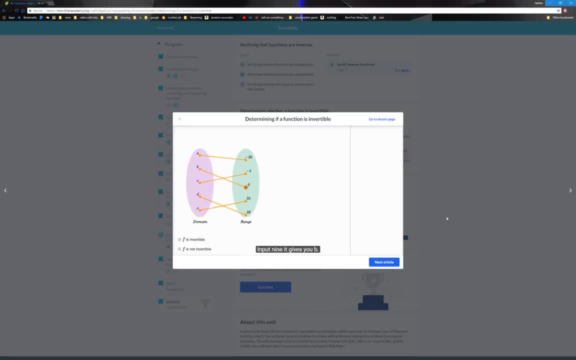 it should give you d- Input 25,. it should give you e- Input 9, it gives you b- You input negative 4 and input c: You input negative 36, it gives you a. So you could easily construct an inverse function here. 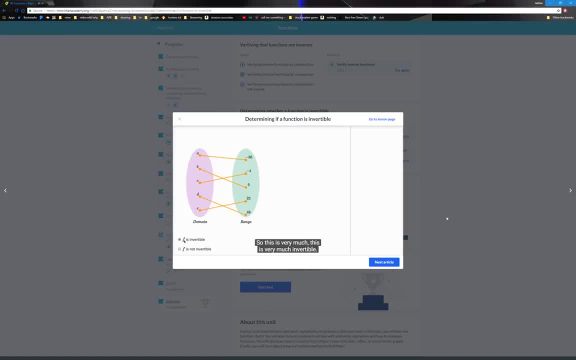 So this is very much. this is very much invertible. One way to think about it is: these are a. this is a one-to-one mapping. Each of the members of the domain correspond to a unique member of the range. You don't have two members of the domain. 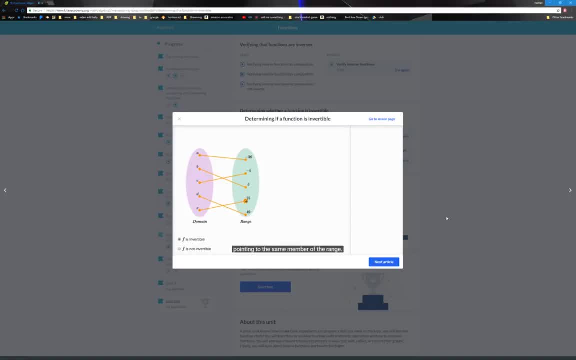 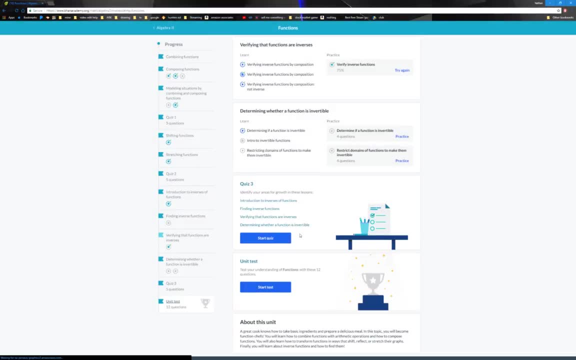 pointing to the same member of the range. Anyway, hopefully you found that interesting. All right, now we're gonna move on to the article, which is yep intro. All right, so here we go. Intro to invertible functions. 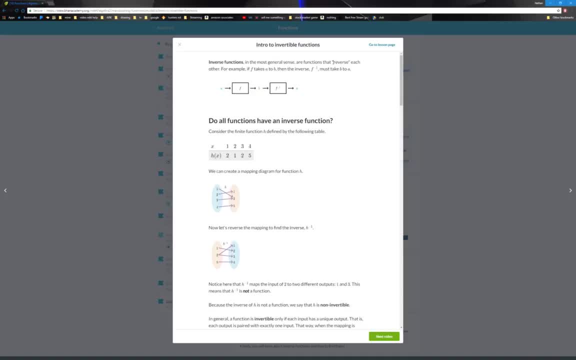 Inverse functions in the most general sense are functions that reverse each other. For example, if f takes a to b and then the inverse- f inverse- must take b to a. So a input into f gives b, b into f. inverse must give a. 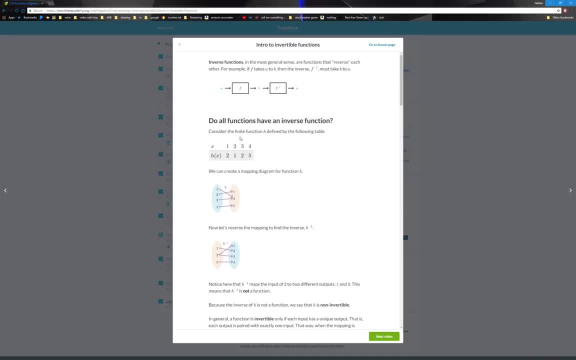 So do all functions have an inverse function. Consider the finite function h, defined by the following table: 1 to 2,, 2 to 1,, 3 to 2, and 4 to 5.. We can create a mapping diagram for function h. 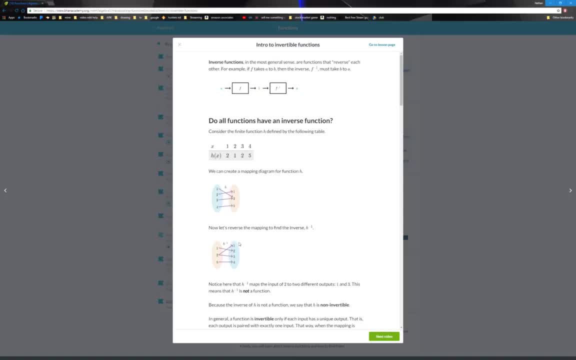 1 to 2,, 2 to 1,, 3 to 2,, 4 to 5.. Now let's reverse the mapping to find h inverse. Well, 1 to 2,, 2 to 1, and 3,. 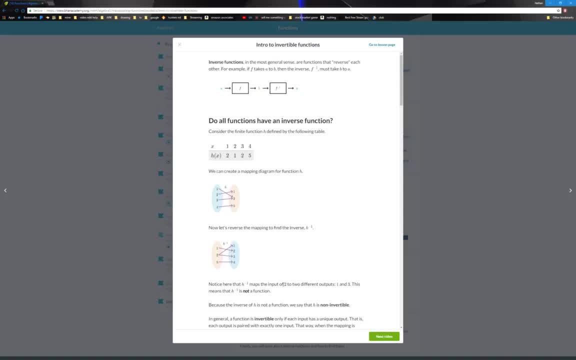 and then 5 to 4.. Notice that h inverse maps two different outputs: 1 and 3.. Two different outputs for the input of 2, 1 and 3. This means that h inverse is not a function, because you can't have one input. 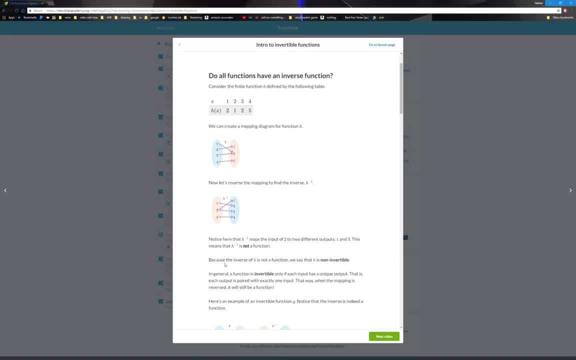 and have two different possible outputs. Because the inverse, h is not a function, we say that h is non-invertible. In general, a function is invertible only if each input has a unique output, That is, each output paired with exactly one input. 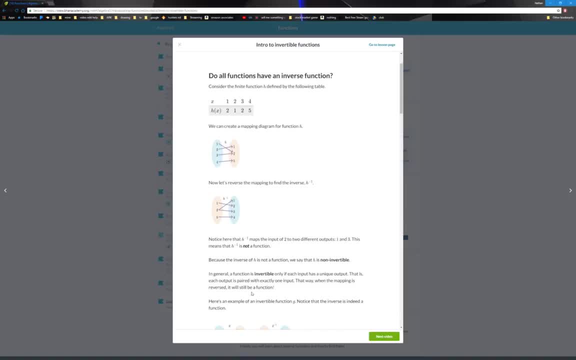 That way, when the mapping is reversed, it will still be a function. Here's an example of an invertible function: g. Notice that the inverse is indeed a function, So 1 to x, 2 to z and 3 to y. 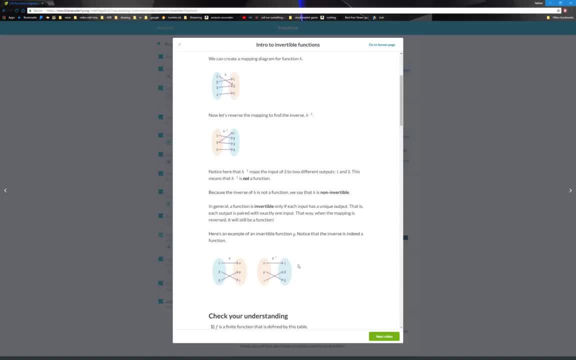 And that's 1 to 1.. Each input has an output, has its own unique output: x to 1,, y to 3, and z to 2.. That's g inverse and it is invertible because no input has more than one output. 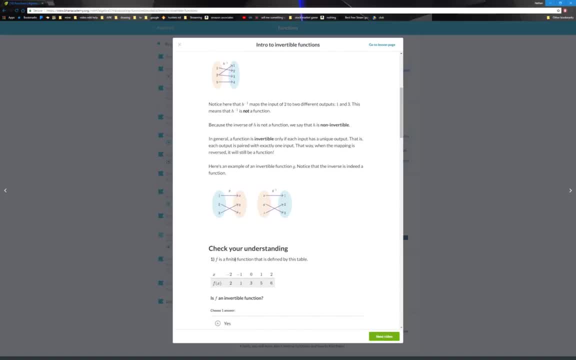 So check your understanding. f is a finite function that is defined by this table: Negative 2 to 2, negative 1 to 1,, 0 to 3,, 1 to 5, and 2 to 6.. 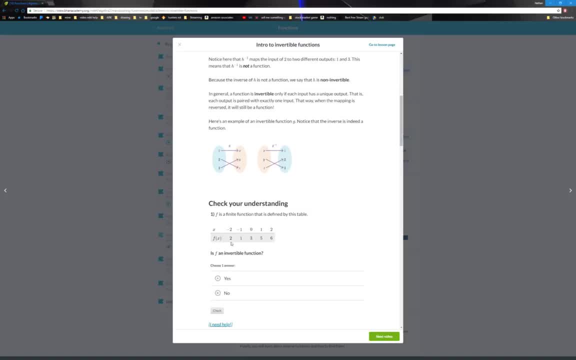 Is f an invertible function? Well, each input has its own unique output that is different from the rest. So, yes, it is an invertible function. g is a finite function that is defined by this table: 2 to negative 2,, 5 to negative 3,. 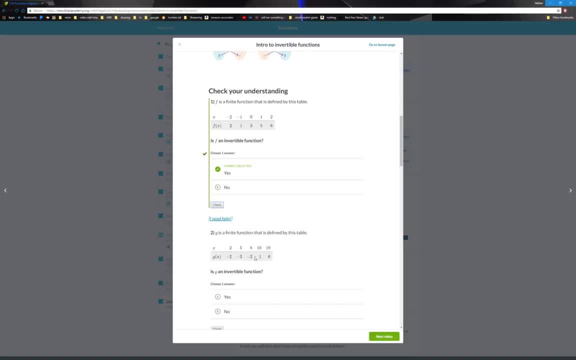 8 to negative 2,, 10 to 1, and 19 to 6.. Is g an invertible function? Well, if we flipped it around: negative 2 to 2, negative 3 to 5, and negative 2 to 8,. 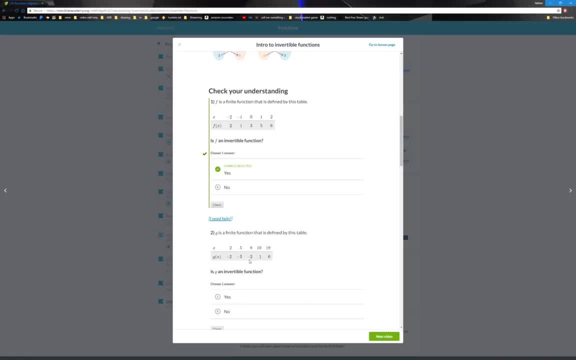 well, there's another negative 2 that has the same output. that has different output. So g is an invertible function. It has a different output than the other negative 2.. So g inverse is not a function. So we got that right. 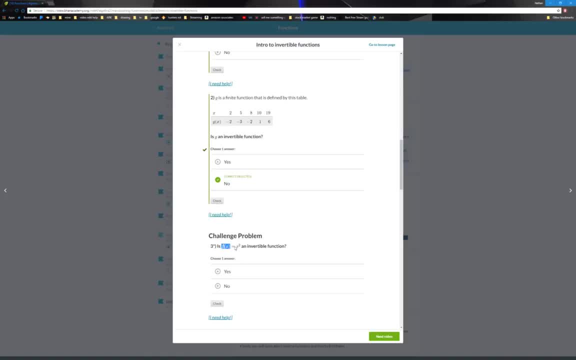 The challenge problem is: f of x equals x squared, an invertible function. So let's think about this. Think of any number you could input like: 0 would give you 0,, 1 would give you 1,, 2 would give you 4,. 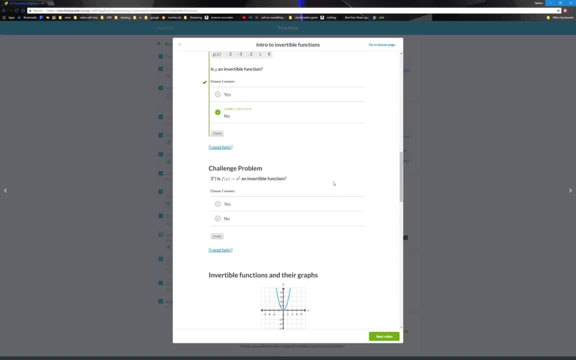 4 would give you 16. So each input has its own unique output. So, yes, and that is not correct. We'll see why. So, oh, I didn't even think about negatives. Every negative number squared is the same thing. 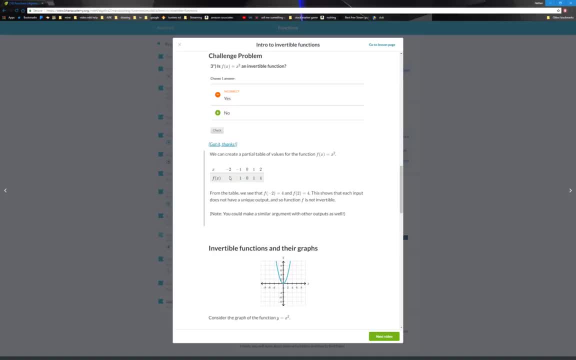 And the inverse. if you input it, you couldn't get a negative um, a negative uh output. So no Invertible functions and their graphs. Consider the graph of the function: y equals x squared. That's this one, right here. 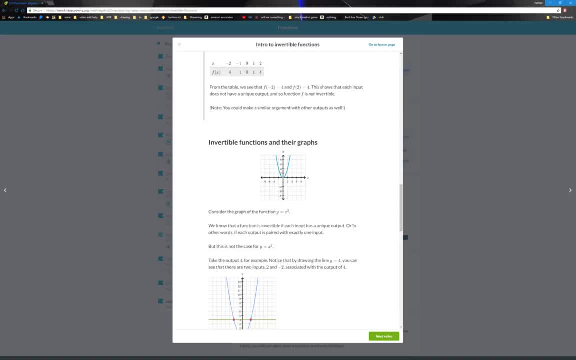 We know that a function is invertible if each input has a unique output, Or in other words, if each output is paired with exactly one input. But this is not the case for y equals x squared, And it shows you down here. 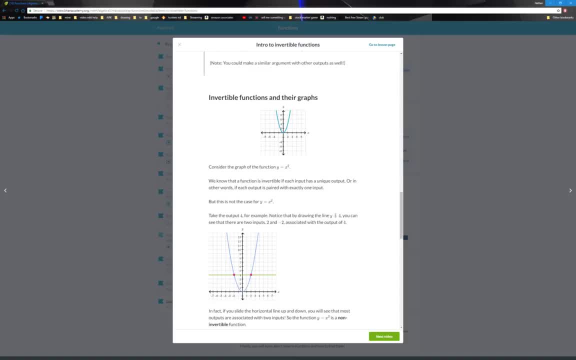 Take the output 4,, for example. Notice that by drawing a line, by drawing the line y equals 4, you can see that the two inputs 2 and negative 2 are associated with the output 4.. And you can do that with any um. 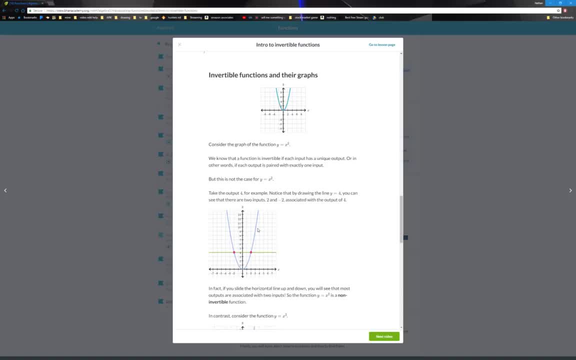 6 is both of these: About 2 and a half-ish 9.. Here is 3 and negative 3. But yet, no matter where you move it, it's got 2 points. So, in fact, if you slide the horizontal line up, 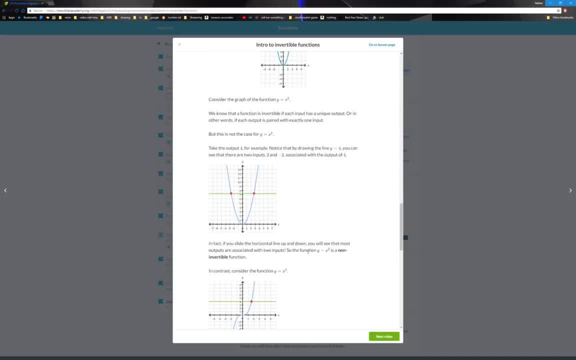 which is what we just did. you'll see that most outputs are associated with 2 inputs. So y equals x, squared is a non-invertible function. In contrast, consider the following: y equals x cubed, As you can see, 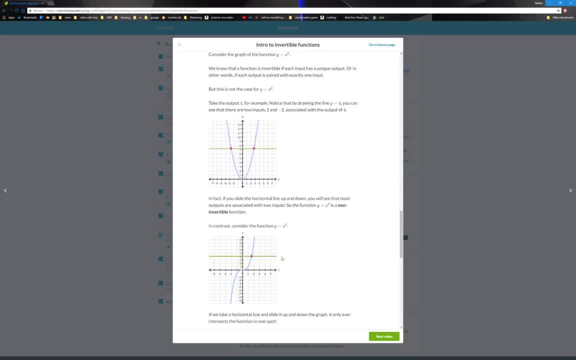 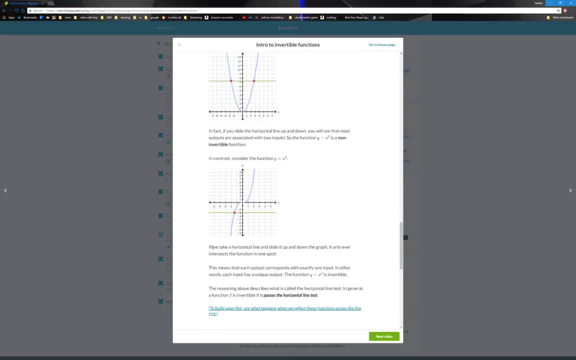 no matter where we slide this horizontal line, it's always on 1 point, not 2.. So this is an invertible function. If we take the horizontal line and slide it up and down the graph, it only ever intersects the function in 1 spot. 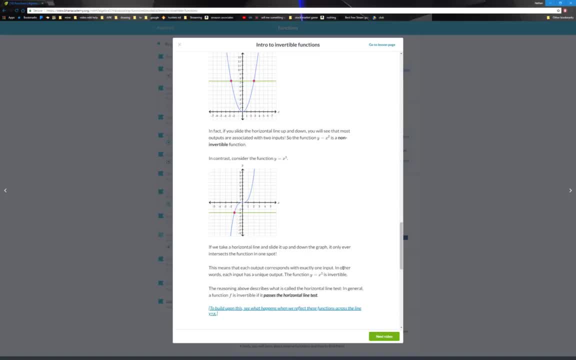 This means that each output corresponds with exactly 1 input. So 1 input along x gives you exactly 1 output along y. The function y equals x. cubed is invertible. The reasoning above describes what is called the horizontal line test. 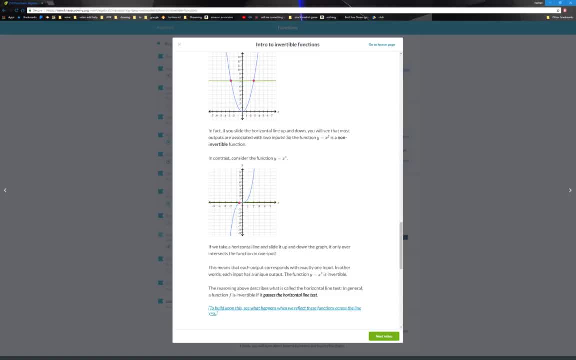 In general, if a function f is invertible, it passes the horizontal line test. To build upon this, see what happens when we reflect across the line y and x. Recall that a function and its inverse are reflections over the line y equals x. 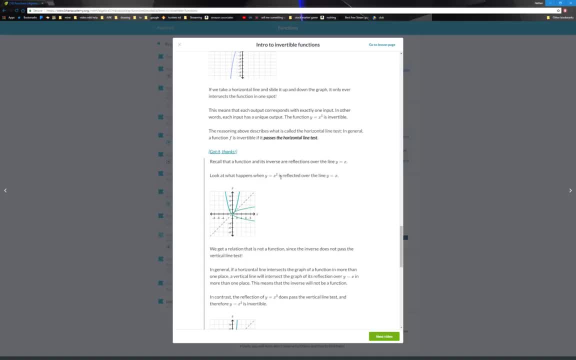 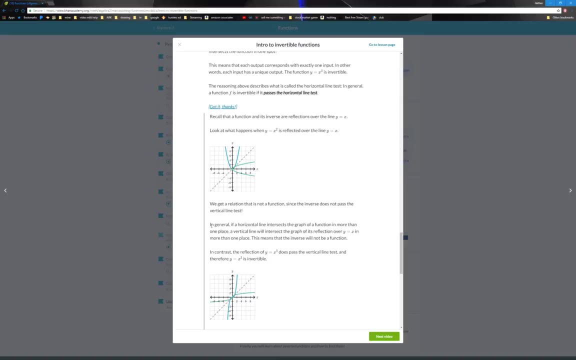 Look what happens when y equals x, squared, is reflected over the line y. We get a relation that is not y equals x. We get a relation that is not a function and the inverse does not pass the vertical line. In general, if a horizontal line intersects. 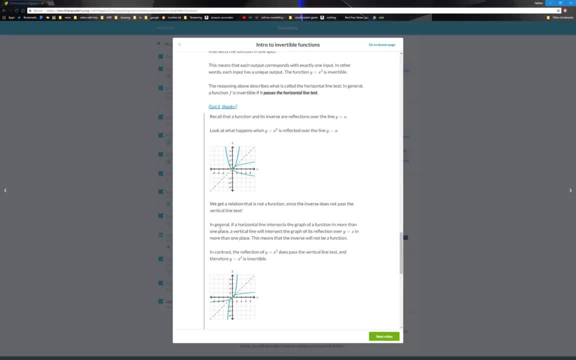 the graph of a function in more than 1 spot, a vertical line will intersect the graph of its reflection over. y equals x in more than 1 place. See how they intersect here twice. In contrast, the reflection of y equals cubed does pass the vertical. 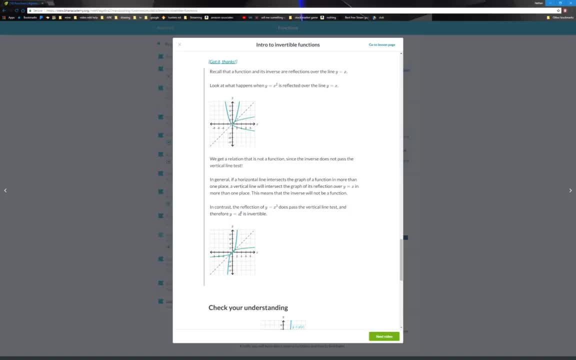 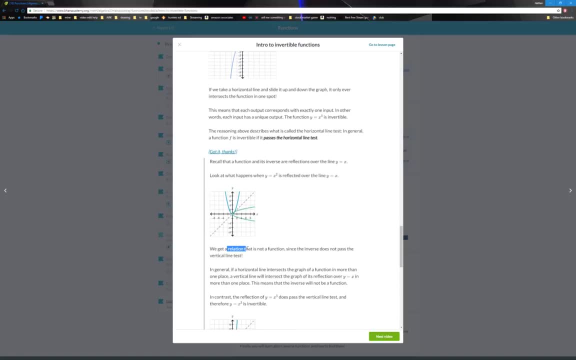 line test and therefore the y equals cubed is invertible. So We'll check our understanding here. Is g invertible? Well, if we took the horizontal line test and we drew a line across Here, there wouldn't be a problem. 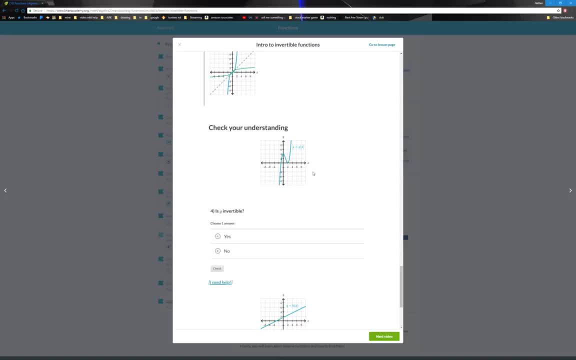 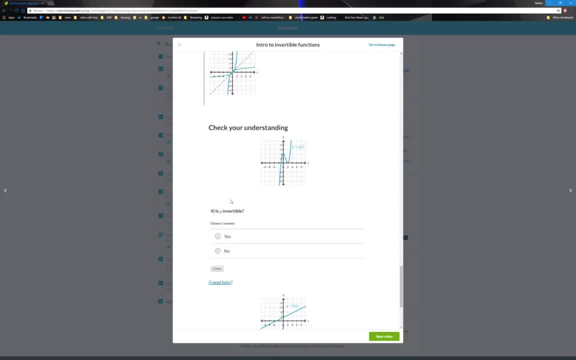 y equals 2, it crosses here, here and here and that's 3.. So These 3 different x inputs would all give you the same y output, which means y output can't give you more than 1 input. so g is not. 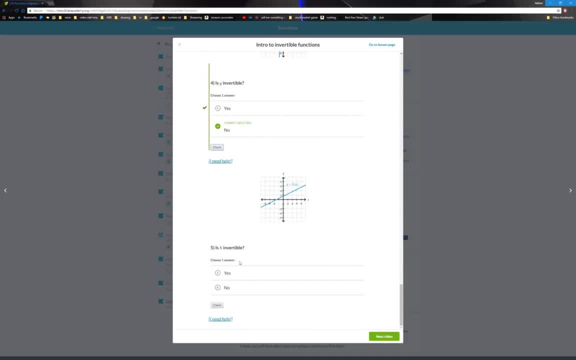 invertible. Now is h invertible? Well, if we did the horizontal line test, we drew a line here, no problems, and we kept sliding it up, it would only ever cross once along this horizontal line. so yes, it is invertible. 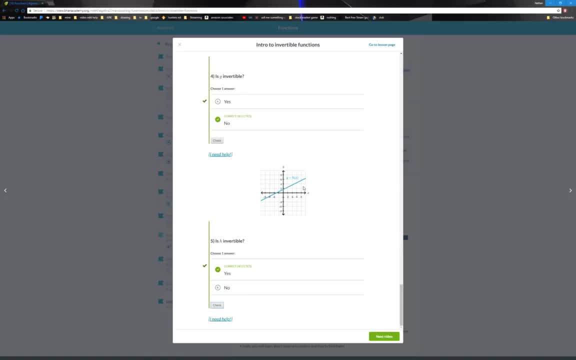 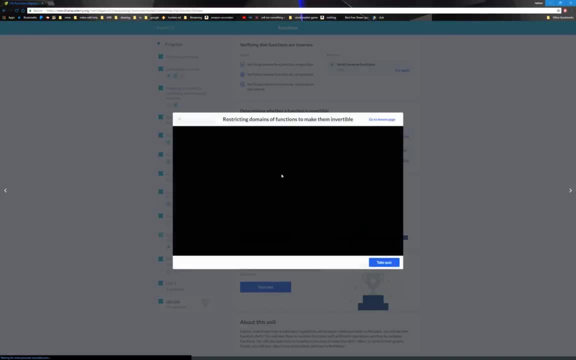 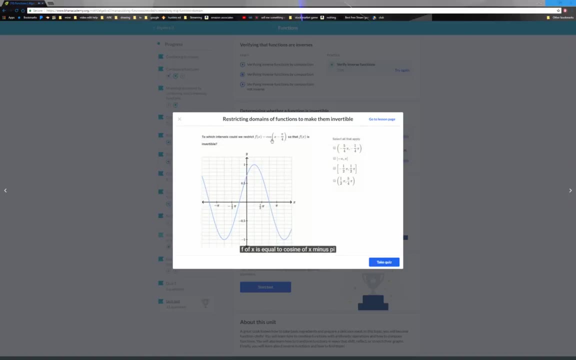 Because each input has its own unique output and each output has its own input. So now we have just a video and then we have some practice problems to do. To which intervals could we restrict? f of x is equal to cosine of x minus pi over 4,. 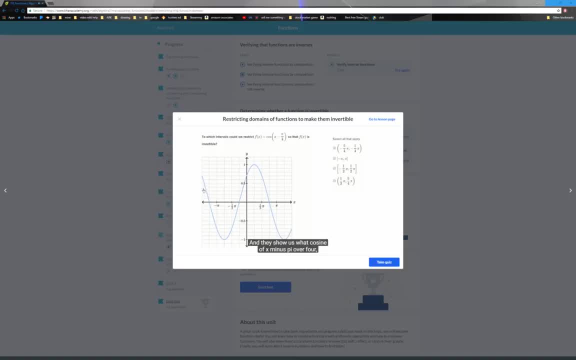 so that f of x is invertible and they show us what cosine of x minus pi over 4, what it looks like the graph of it. So let's just think about what it means for a function to be invertible. So a function is a mapping from a set of. 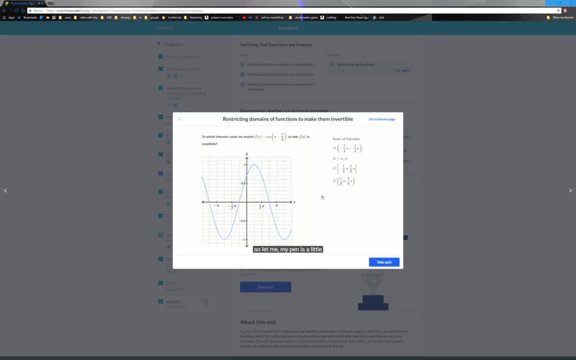 elements that we would call the domain. So let me- my pen is a little off today, so let's see if it works, okay. So this right over here is our domain and this over here is our range. Our range And a function maps from. 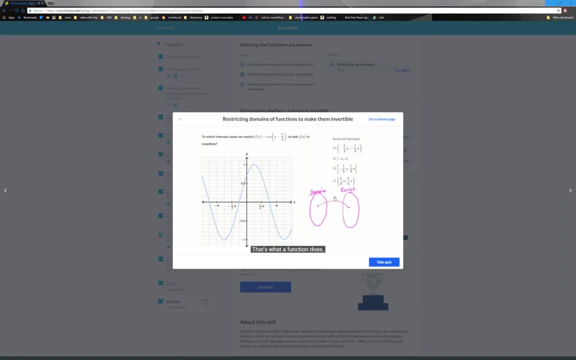 an element in our domain to an element in our range. That's what a function does. Now the inverse of the function maps from that element in the range to the element in the domain, So that over there would be f inverse. So that's the. 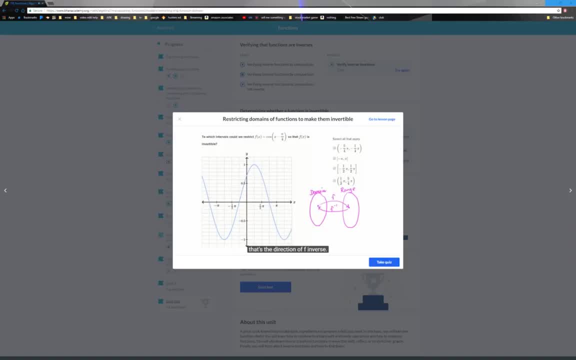 direction of the function, that's the direction of f inverse. Now, a function is not invertible. One of the situations in which a function is not invertible, you could have a function where two elements of the domain map to the same element of the range. 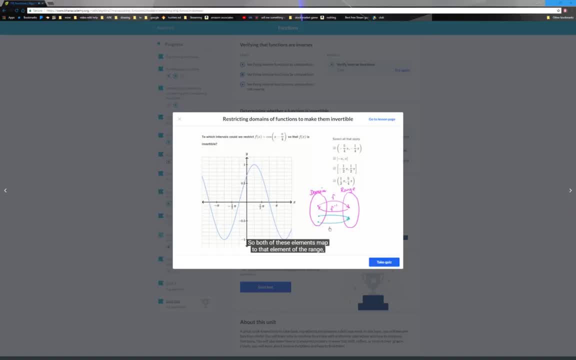 So both of these elements map to that element of the range. So both of these are the function. But then, if this is the case- it's going to be- you're not going to be able to create a function that maps the other way, Because if you input, 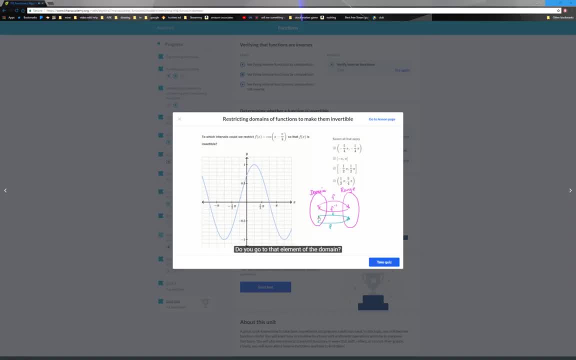 this into the inverse function: where do you go? Do you go to that element of the domain, Or do you go to that element right over there? And so one way to think about it is you need a one-to-one mapping for each element of. 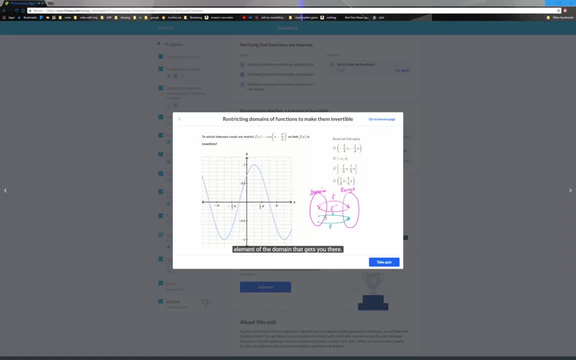 the domain range. There's only one element of the domain that gets you there. Or another way to think about it: you could try to draw a horizontal line on the graph of the function and see if it passes, if it crosses through the function more than once And you 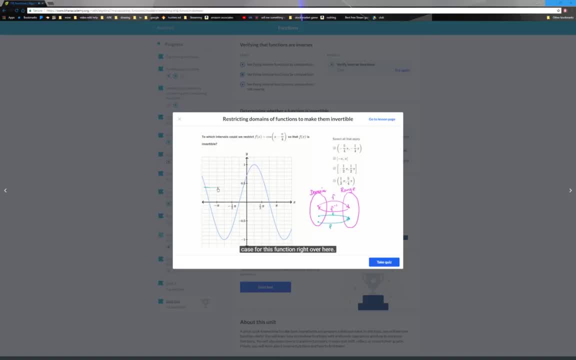 could see that this is indeed the case for this function right over here If I did a horizontal line right over here. Now, why is this the issue? Well, this is showing us actually. let me do a number that's a little bit easier to look at. So let's say I drew. 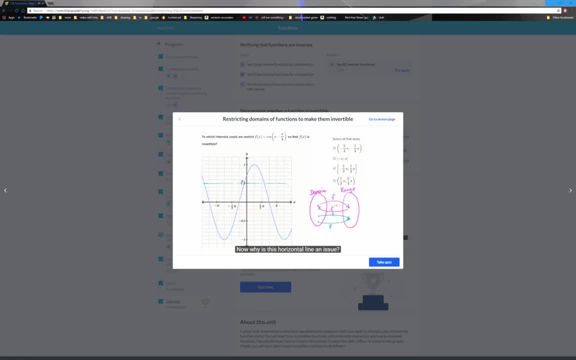 the horizontal line right over here. Now, why is this horizontal line an issue? Well, it's showing us that just even the part of the domain that's being graphed here, that there's several points that map to the same element of the range. They're mapping to 0.5.. 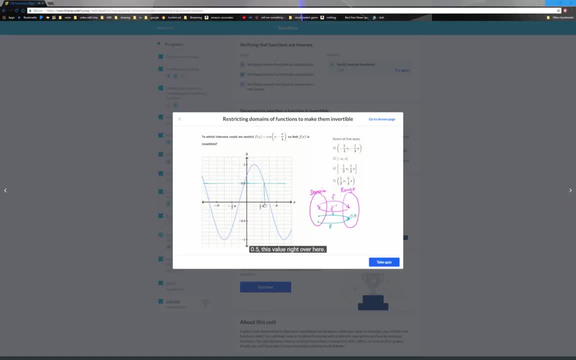 0.5.. 0.5.. If you this value right over here when you take, when you input f of that is equal to 0.5.. f of this right over here is equal to 0.5.. 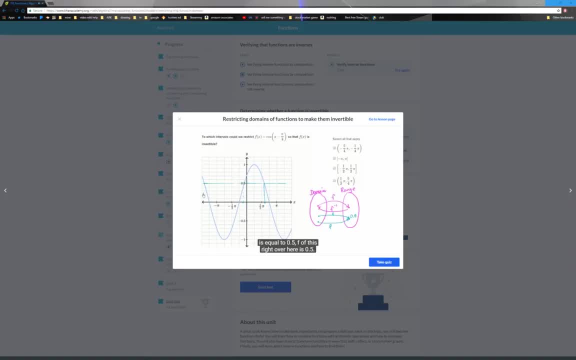 f of this right over here is 0.5.. So if you have that, if you have multiple elements of your domain mapping to the same element of the range, then the function will not be invertible for that domain. So really, what we're going to do is we're going to try to restrict. 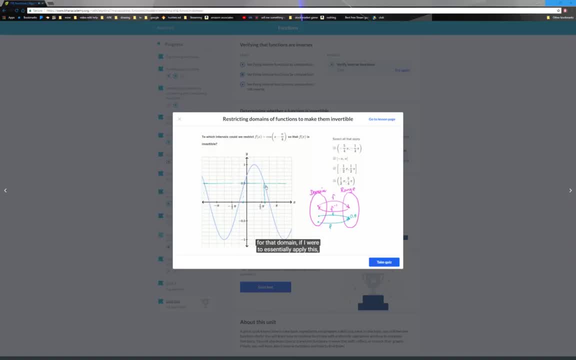 the domain, so that for that domain, if I were to essentially apply this, what I'd call the horizontal line test, I'd only intersect the function once. So let's look at the or the graph of the function once. So let's look at these choices. 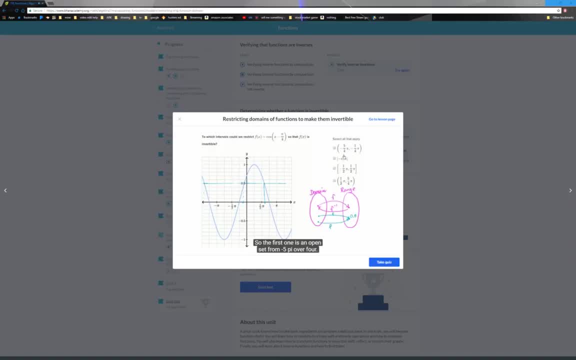 So the first one is an open set from negative 5 pi over 4.. Negative 5 pi over 4.. So that's pi, that's negative pi and another fourth of pi. So that's, I think, starting right over here, Going all the way to negative. 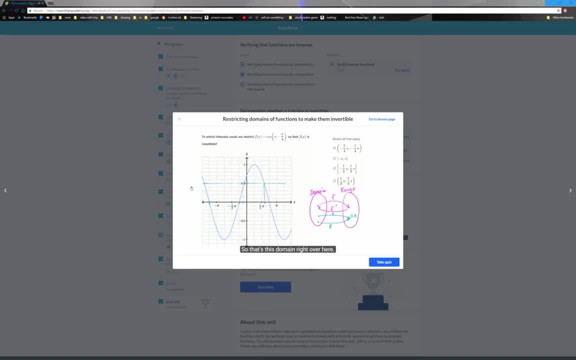 one fourth pi. So that's this, this domain, right over here. Let me do this in a new color. So that's this. And this does not include this does not include the two endpoints. So here I can still apply the horizontal line and in that domain. 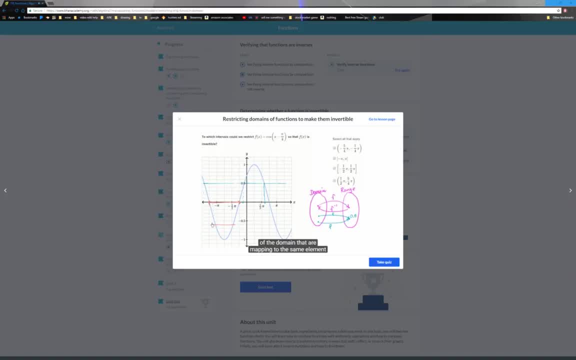 I can show that there's two members of the domain that are mapping to the same, to the same element in the range, And so if I'm trying to construct the inverse of that, what would that, which I guess is negative 0.6? what would that f inverse of negative 0.6? 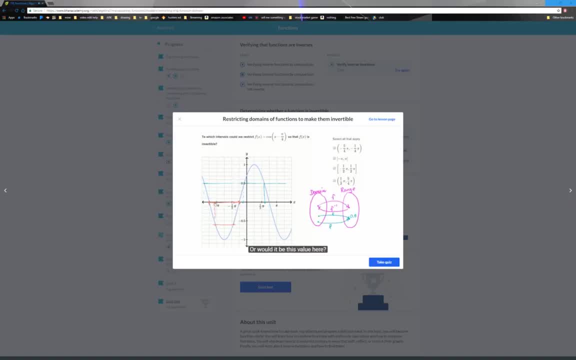 be. Would it be this value here or would it be this value here? So I would rule this one out. So let's see Negative pi to pi. So negative pi to pi. I'll do this in. I'll do this in this color. 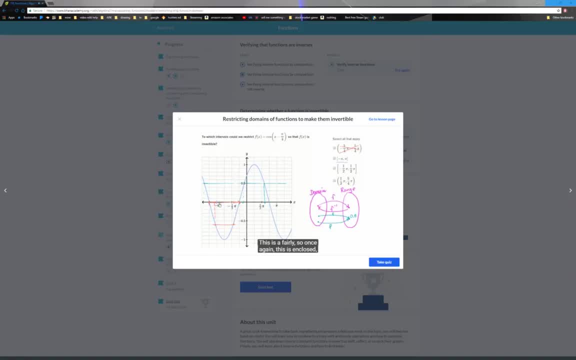 right over here. Negative pi to pi. This is a fairly So once again over this is a close. so we're including the two boundaries, We're including negative pi and pi in the domain, But once again, over that interval I could apply my horizontal line here. 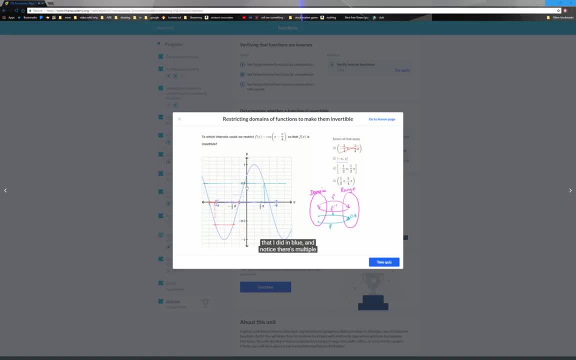 and notice, or actually I could even apply the original one that I did in blue and notice there's multiple elements in the domain that map to say 0.5. So what would f inverse of 0.5 be? You can't construct a function. 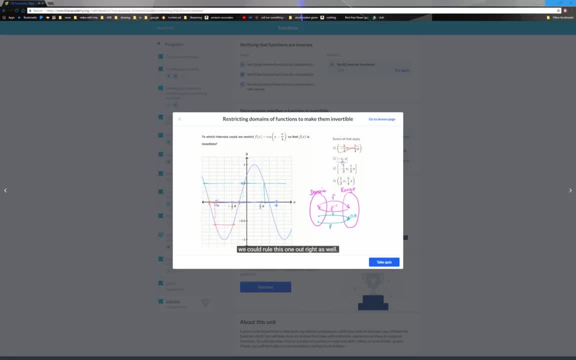 where it maps only to one element of the domain. So we could rule this one out right as well. Now, negative 1 half pi to positive 1 half pi. So negative 1 half pi. so that is so, let me. I'm running out of colors. 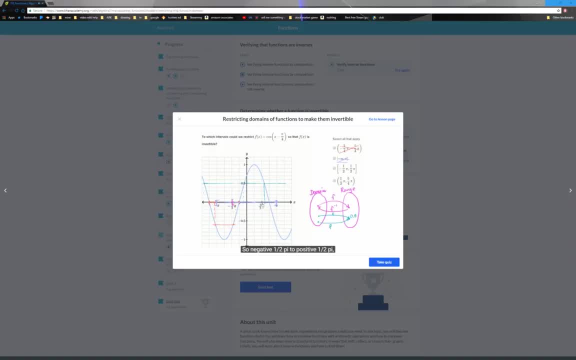 so negative 1 half pi to positive 1 half pi. this one is interesting if I apply a horizontal line there, there, there. so let's see. but if I apply a horizontal line right over here, I do intersect the function twice. so I have two members. 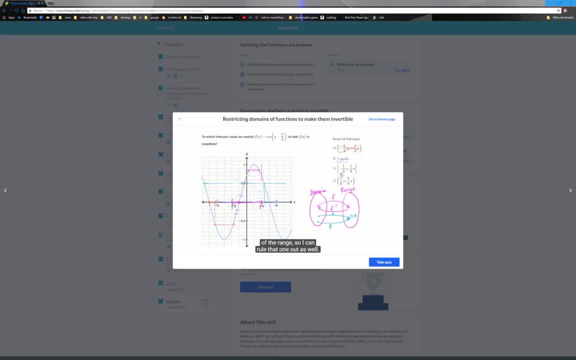 of this domain mapping to the same element of the range. so I could rule that one out as well And I'm left with one last choice, so I'm hoping this one will work out. So 1 half pi, since it's an open set. 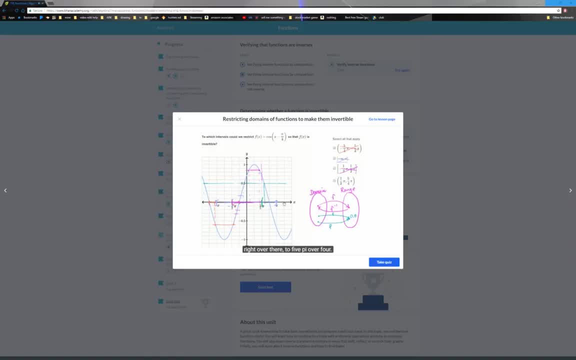 so 1 half pi right over there to 5 pi over 4.. 5 pi over 4.. So that's pi, and another 1 fourth, so that's right over there, and let's see this is. if I were to look at the graph here, it seems like it would. 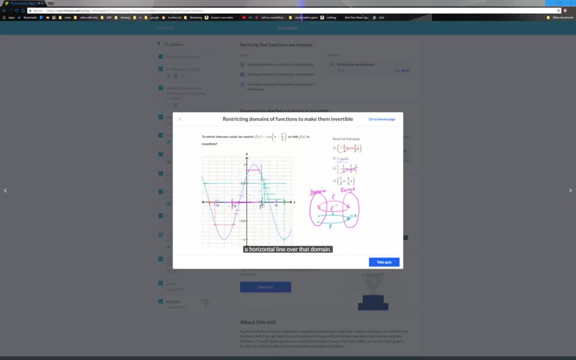 pass the horizontal line test At any point here, I could make a horizontal line over that domain. Actually, let me do it for the whole domain. so you see that for the whole domain and I'm only intersecting the function once. So for every element of 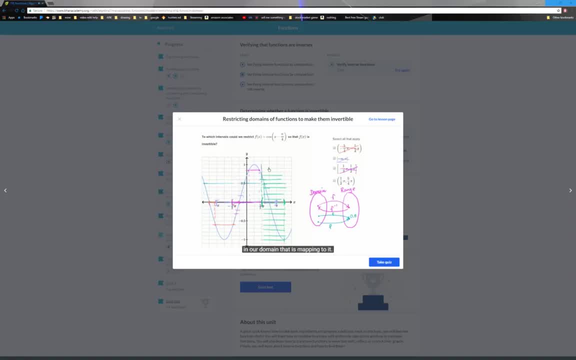 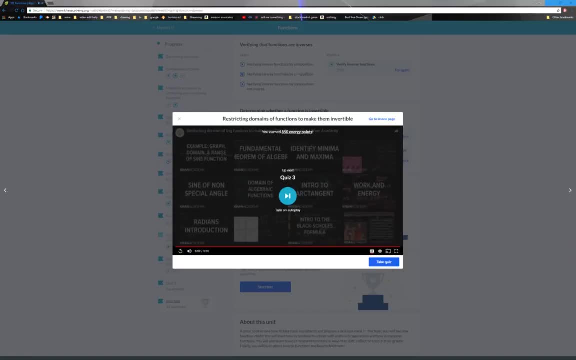 the range that we're mapping to. there's only one element in our domain that is mapping to it. It's passing our horizontal line test, so I would check this one right over there. Alright, now we're going to move on to do the practice problems. 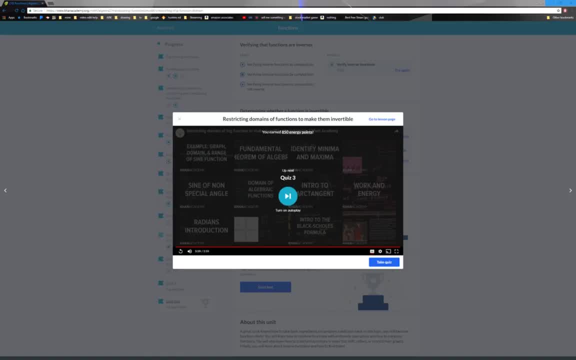 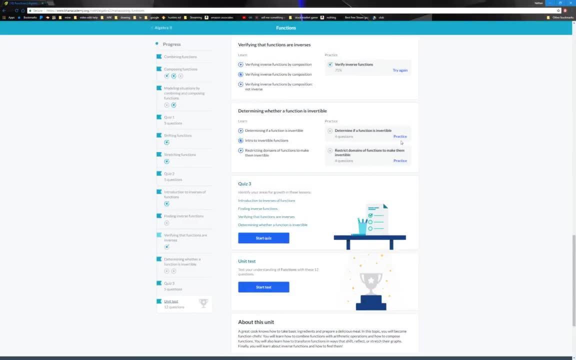 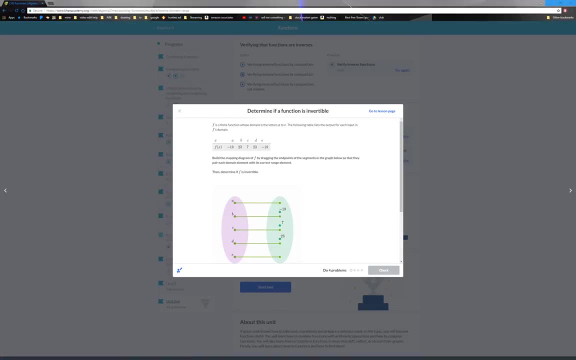 There we go, Alright. So determine if a function is invertible: practice, There we go. One sec, Alright. Alright, here we go. Had to get some stuff re-arranged. Had to get some stuff re-arranged. Had to get some stuff re-arranged. 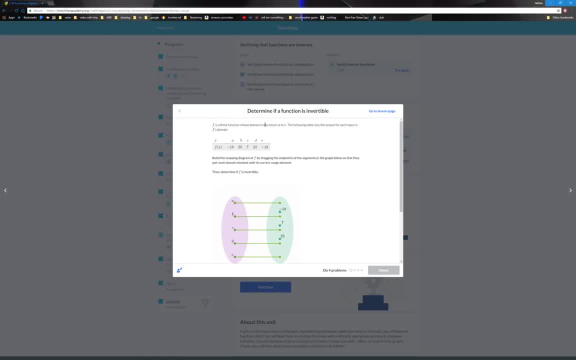 f is a finite function whose domain is the letter a to e. The following table lists the output for each input, for each input in f's domain. So it's x to f of x, a to negative, 19, b to 23, c to 7, d to 23. 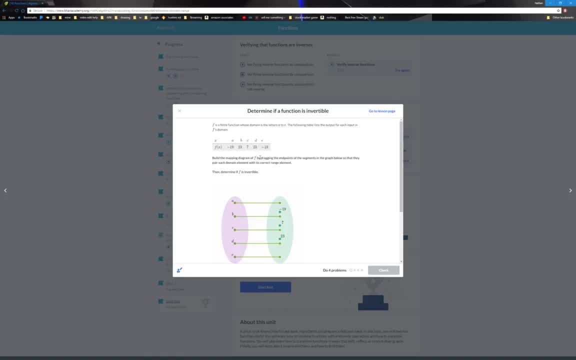 d to 23 and e to negative 19.. Build the mapping diagram for f by dragging the endpoint segments to the graph below so that each domain element pairs each domain element with its correct range element. So a to negative 19, b to 23. 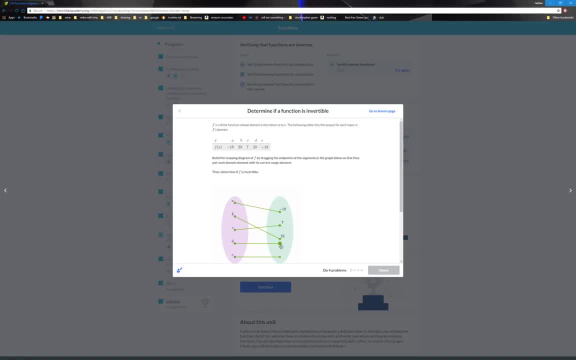 c to 7, d to 23. c to 7, d to 23, 19.. There we go. So choose one answer: F is invertible or F is not invertible. Well, we can see here: A goes to negative 19 and E goes to negative 19.. So that's already one output. 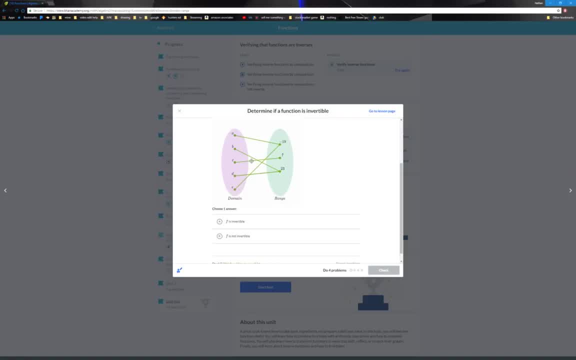 that already has two inputs And 23,. B goes to 23 and D goes to 23.. So that is another output that has two inputs. But just knowing that one output has more than one input, we know that F is not invertible. So F is a finite function whose domain is the letter A to E. 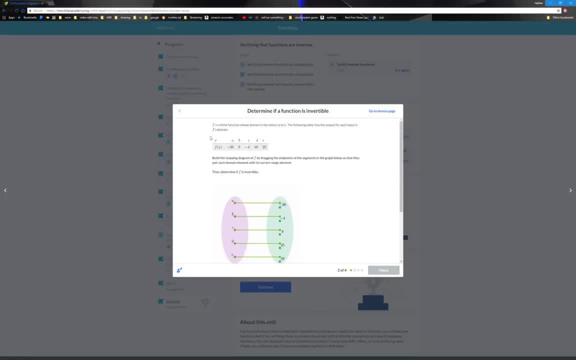 Following: the table lists the output for each input of F's domain. So it's the same thing. We have to drag the endpoints to finish this table. So A to negative 36, B to 19,, C to negative 4,, D to 49, and E to 25.. Now is F invertible, or is it not invertible? Well, 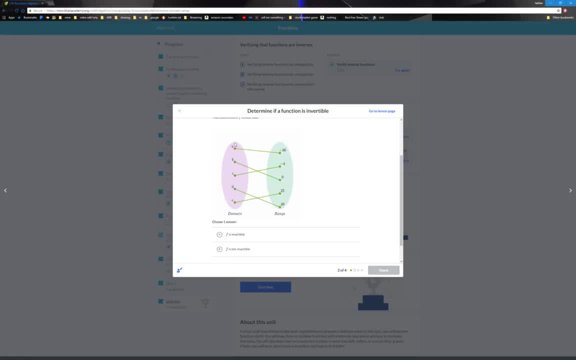 we can look at over here. This negative 36 goes to A, So that's one output. So that's fine if we flip them. If negative 4 was the input, C would be the output. That's only one. So we're fine there. 9 to B: we're fine there, 25.. 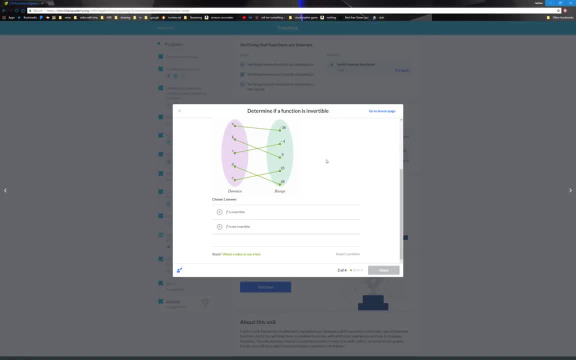 To only E, we're good, And 49 to only D, we're still good there. So F is invertible in this case. So now we have to graph another one: A to 1, B to 2, C to 3, D to 2, and no D to 1,. 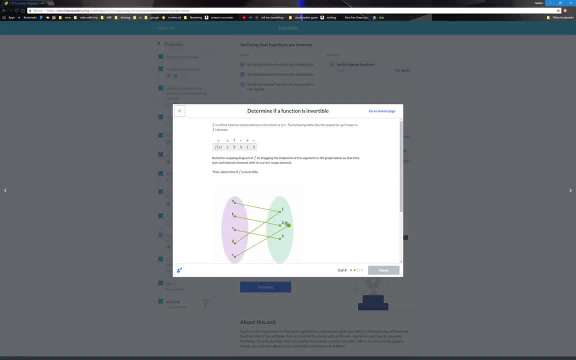 and D to 1.. E to 2.. So is F invertible or not invertible? Well, we can tell here. With 3, we only have one output, So we're fine there. But 2, we have B and E. for the inverse, This would be two. 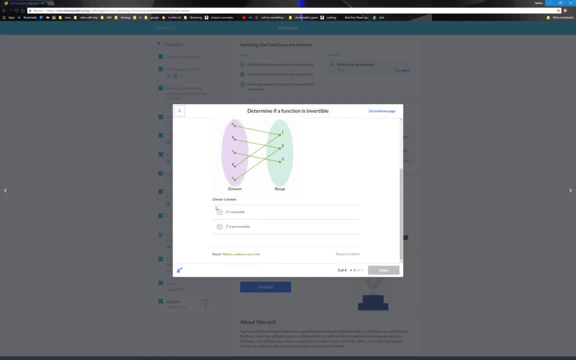 outputs for 1. And for 1, we'd also have two outputs. So that is not possible. So F inverse is not a function. So now we have another one: A to 11. B to 15. C to 9.. 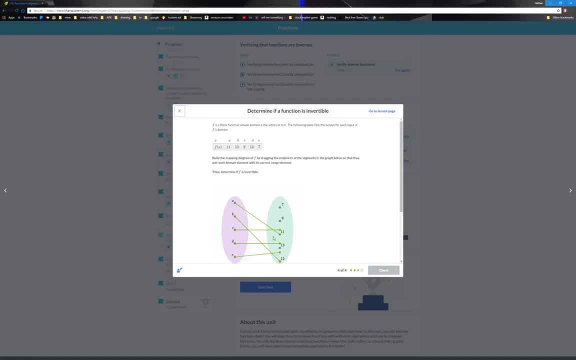 E to oh, C to 9.. D to 13. And E to 7.. So now we have to figure out if F is invertible. Well, 15 only goes to B, 13 only goes to D. So we're good. 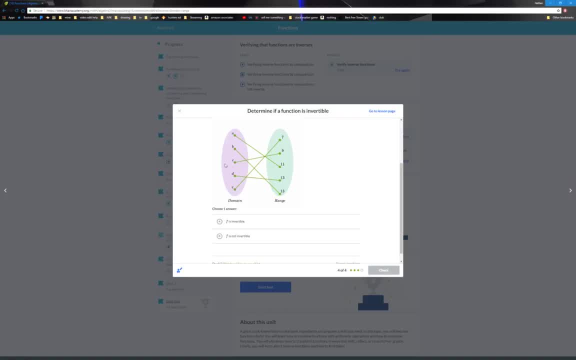 And both of those. 11 only goes to A, That's OK. 9 only goes to C, We're good. And 7 only goes to E, And in this case F is invertible because each output has its own input. 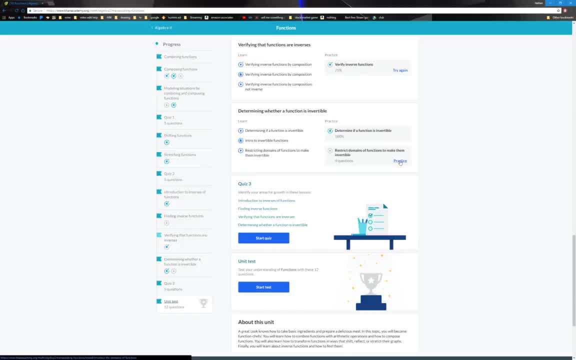 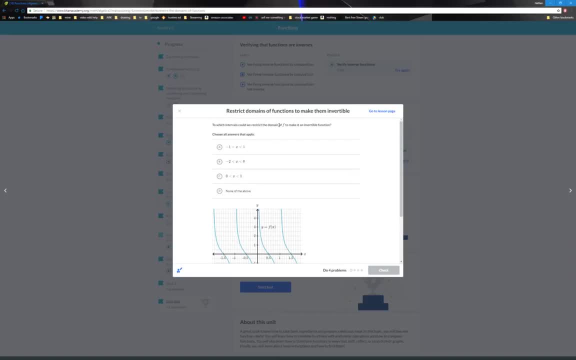 So now we have restrict domains of functions to make them invertible. So to which intervals could we restrict the domain of F to make it an invertible function? Choose all that apply. So X has to be greater than negative 1, but less than 1.. 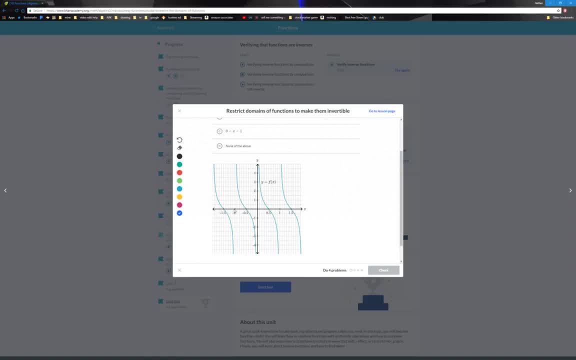 So X be greater than negative 1.. That would be along this line here, Greater than negative 1, all the way down, All the way down, I guess that's where it stops, But less than 1.. Well, we can see here if we did the horizontal line test anywhere, here, for example. well, 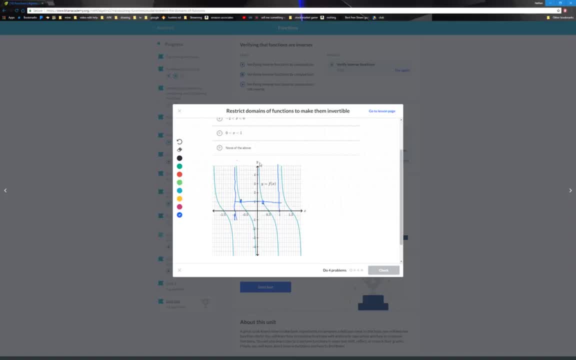 we have two points that are along the same y-axis. So that can't be it. So we know that it's not this one. What about negative 2 to 0?? So negative 2 would be here. Very edge, Very edge to 0, right here. 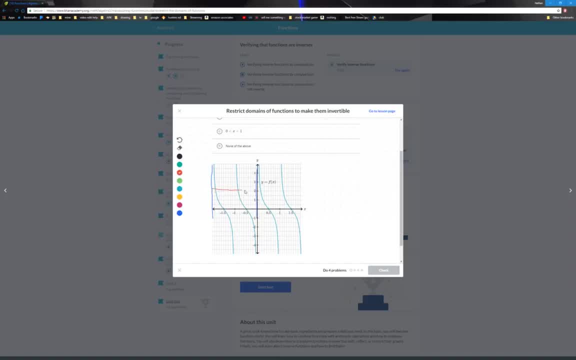 Well, if we did a horizontal line test across anywhere, we could tell that it has two points here, So we know that this one is not it. So what about between 0 and 1? 0 here And 1 here. 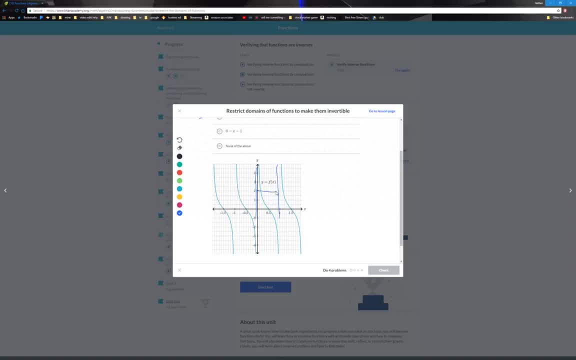 0 here, 0 here. Well, if we did the horizontal line test along the entire thing, we would find that each horizontal line only has one point on it between those two. So we know that that last one will work, And so we'll select it. 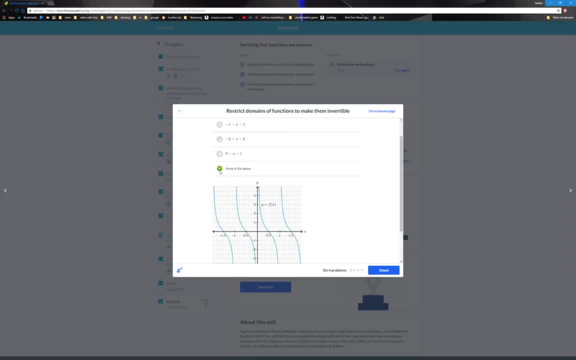 Check. Oh no, no, That is the wrong one. That is the wrong one, Not that one. That is the wrong one. That is the wrong one, That is the wrong one. So we'll do that one. We'll check our answers. 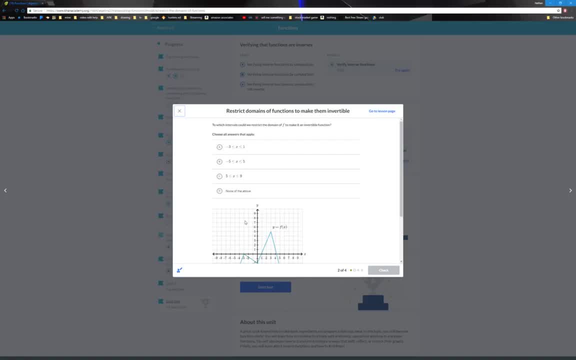 And we got it right. So to which intervals could we restrict the domain of f to be an infertile function? Same thing here. Well, let's check the first one. Negative 3 is less than or equal to x is less than or equal to 1.. 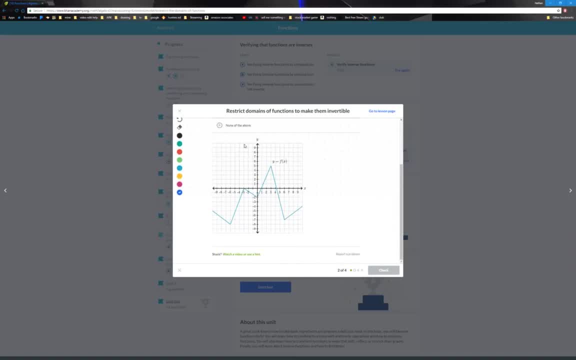 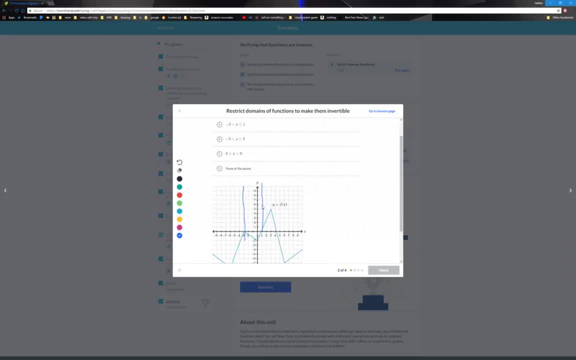 Negative 2 is less than 1.. Oh, that line is so wiggly. And 1. Well, if we did the vertical line test here, we would find that there are two points that cross this vertical line. so we know that this one 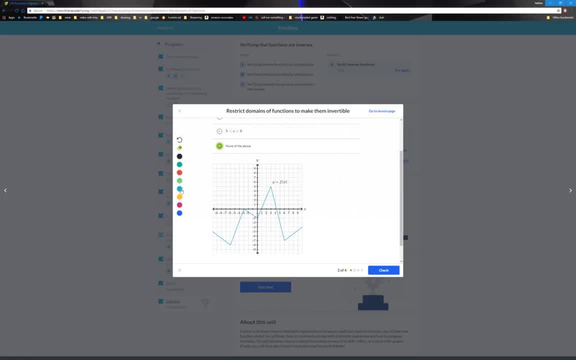 And if I could just un-highlight those, We know that that one is not it, So now we'll try the next one. b. So negative 5 is less than or equal to x, less than or equal to 5.. Negative 5, less than or equal to x, less than or equal to 5.. 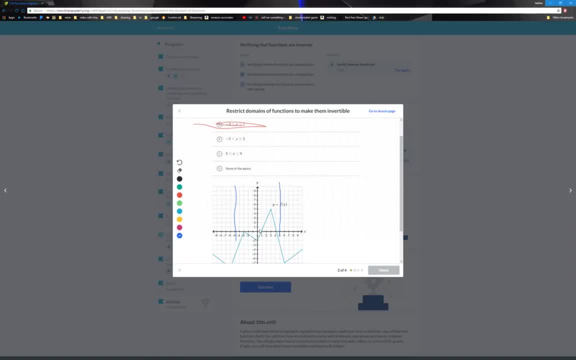 Well, since this one before fit inside of this equation, and it did have a line that was intersected twice, this one is actually bigger and intersects four times. so we already know that, since this one was inside of that, we know that this can't be the answer. 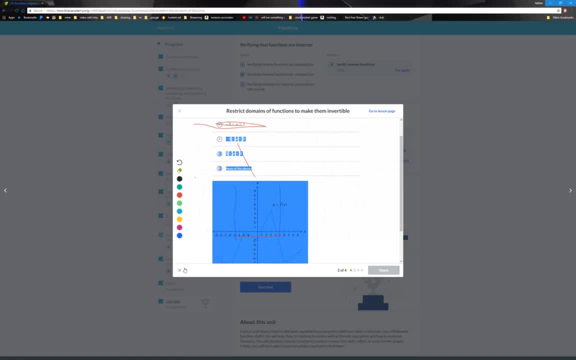 If I could, just So we know that this one can't be it. What about between 5 and 9? 5 and 9.. Well, if I could draw one all the way down to here, I'm going to draw them all the way down. 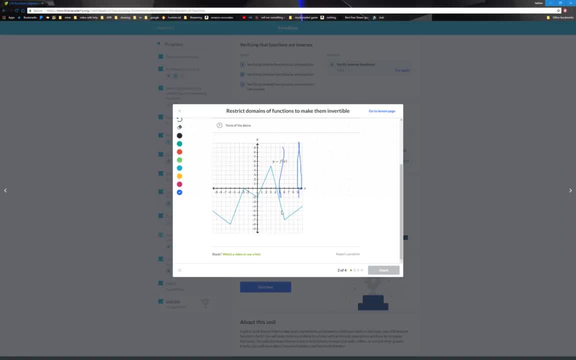 and then we drew a horizontal line across here, we'd see that it intersects. Well, if we did it here, it'd intersect here and here. If we did it lower, it'd intersect here and here. So we know that this one can't be it either. 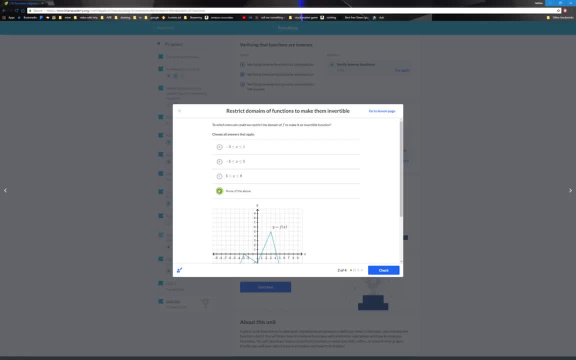 So we know that the answer has to be none of these, And we'll move on to the next question. Okay, To which intervals Could we restrict the domain of f to make it an invertible function? Choose all answers that apply. Well, we could restrict the domain of f to make it an invertible. 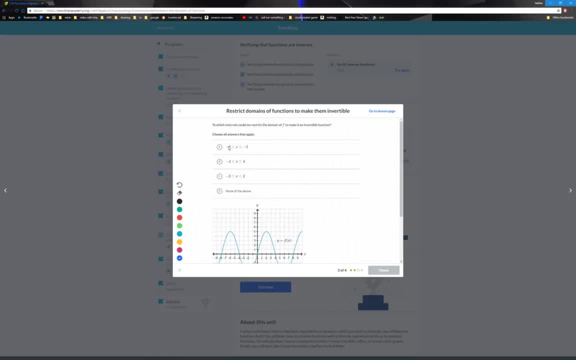 So we're going to test the same exact thing. So, between negative 6 is less than or equal to x, which is less than or equal to negative 2? So negative 2 here and negative 6 here. Well, if we followed negative 2 all the way down, 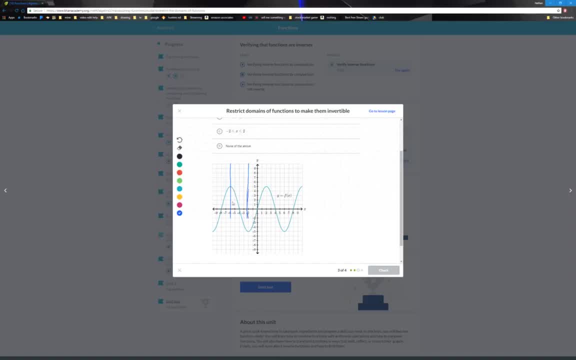 we'd see that it's less than or equal to x, We'd see that it stops here. If we followed 6 all the way up, we'd see it stops here. And if we drew a horizontal line across anywhere, we would see that nowhere does it cross more than one time. 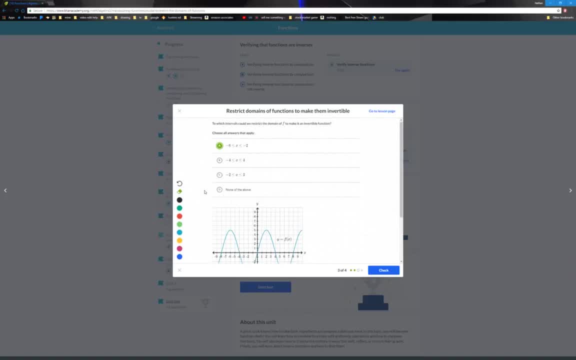 So we know that this one is an answer. So now we're going to try, but we have to select all answers that apply, So it's not going to be just one all the time. So negative 4, negative 4 here and 4 right here. 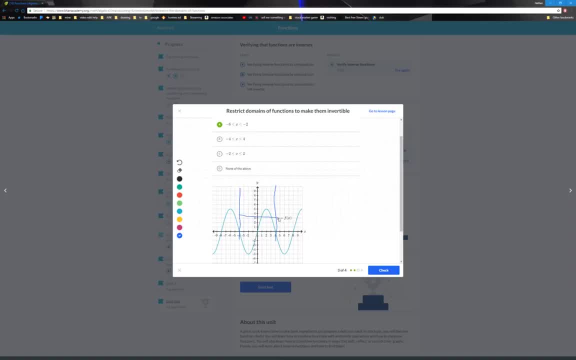 Well, if we drew lines across here, for example, we would see that it intersects here and here, which is two points, which means that this one input has more than one output, which means that that output, That output, if it was an input in an inverse, couldn't equal more than one. 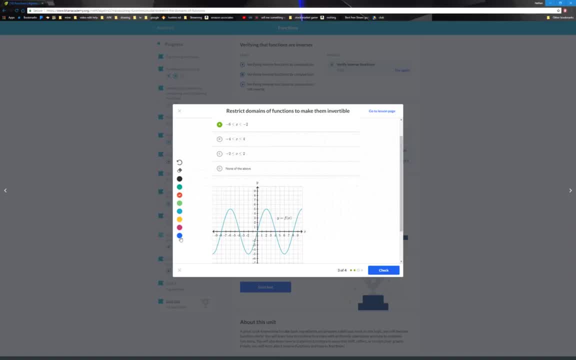 So we know that between these two that won't work. You can draw a line through it Now between: negative 2 is less than or equal to x. negative 2,, which is less than or equal to 2, positive 2.. 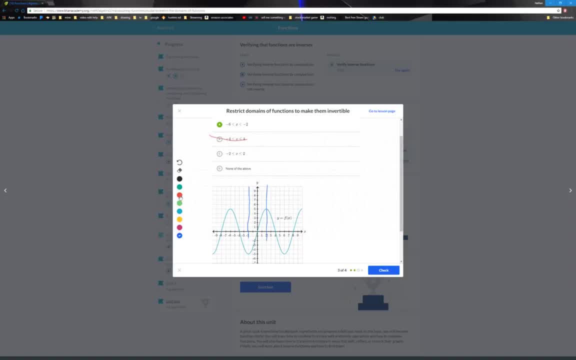 Here we go. So we'd check with the horizontal line test and we'd go all the way across, all the way down. We'd see that nowhere on this does it cross more than once. So we know that this is also an answer. 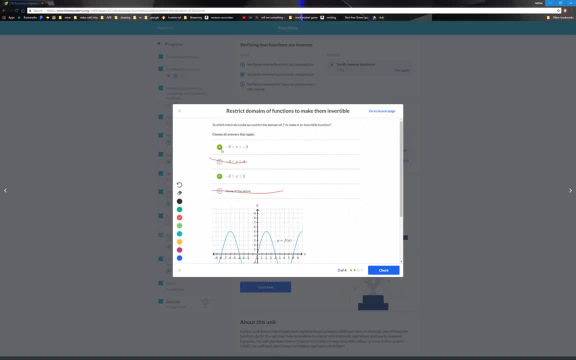 Well, we know that it's not none of these, because we already have two of them selected. So we'll check our answer and we got it right and we'll move on to the last question, To which internet is the internet? 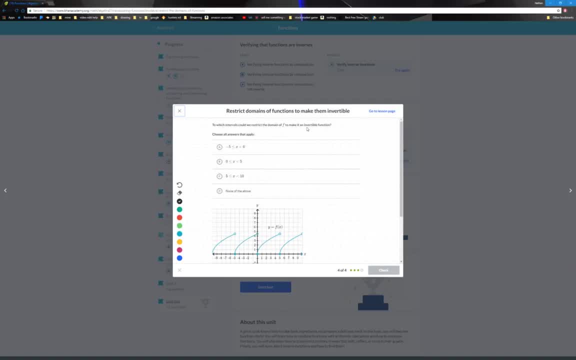 Which intervals could we restrict the domain of f to make it an invertible function? So same thing between negative 5 is less than or equal to x, which is less than 0,. negative 5 is less than or equal to x, which is less than 0.. 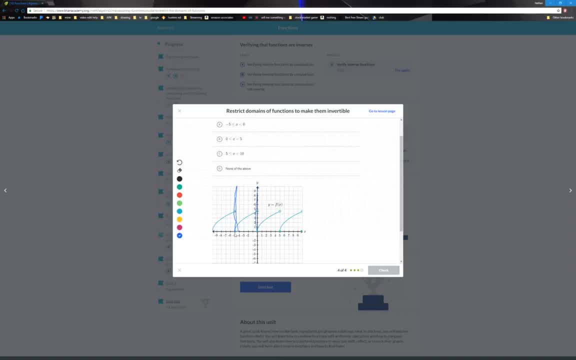 Well, we know that this is not a point because it is open, but this is a point, so we'll just do the horizontal line test And up here all the way down we'd see that nowhere does. are there two points on the same y axis? 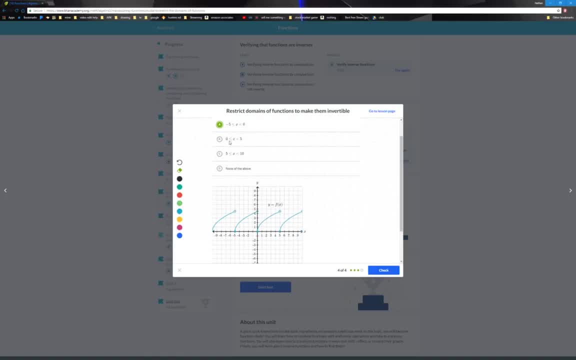 So we know that this is an answer. So between: 0 is less than or equal to x is less than, which is less than 5.. So 0 is less than or equal to x, which is less than 5.. Well, this is a very simple answer. 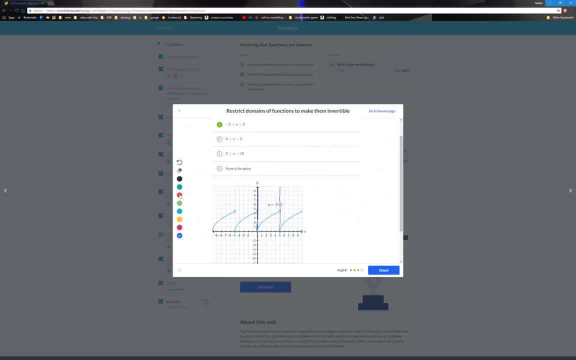 It's a very simple answer. It's a very simple answer. It's a very simple answer. So this, if you look at it, you may think these two points are both there, but we want something less than 5.. This point is on 5, and we would. we're looking for less than 5.. 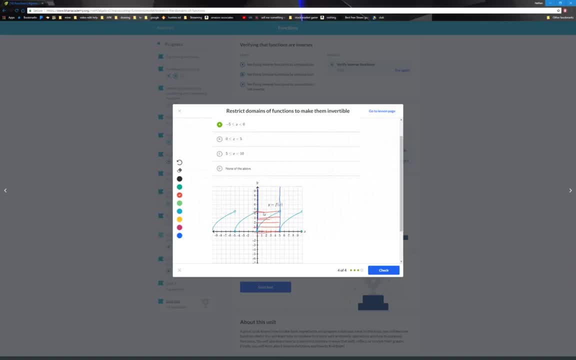 Less than 5.. So we see, and you may see, these two points, but these are both not points that are on the line but less than signs for the graph. So we see that there are no two that cross, no two points that are on the same axis. 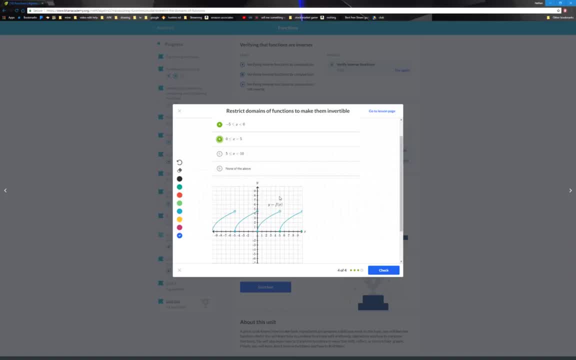 Okay, So we know that this is one. Now, between now, 5 is less than or equal to x, which is less than 10, less than 10, which is here. Well, we know, if we look and we check our horizontal line test, we see once again that 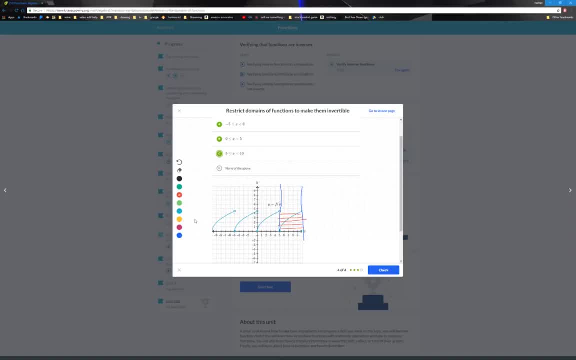 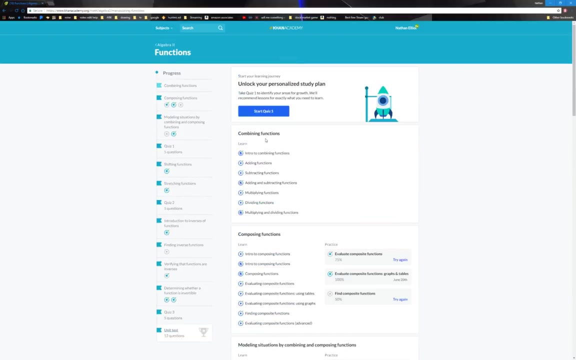 no two points cross the same y axis. There are no. There's no y axis that has two points crossing. So all of them, and we check and we got them all right. So that is determining whether a function is invertible in Algebra 2 in Khan Academy. 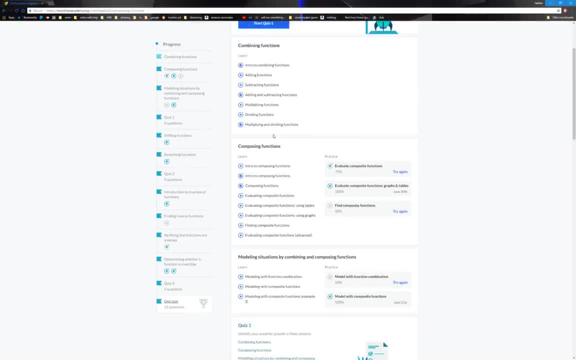 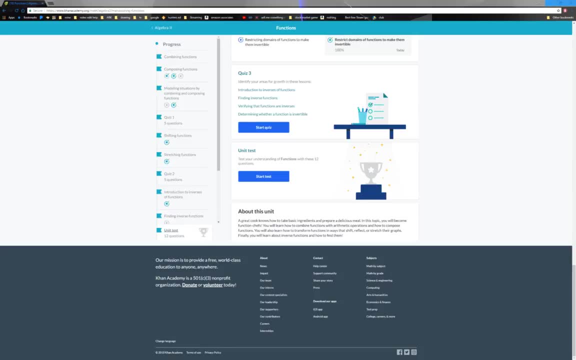 And that's all. and that is all of functions done. So thank you guys for watching and that's all.